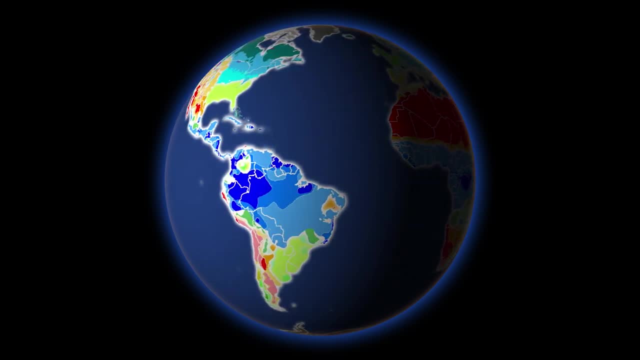 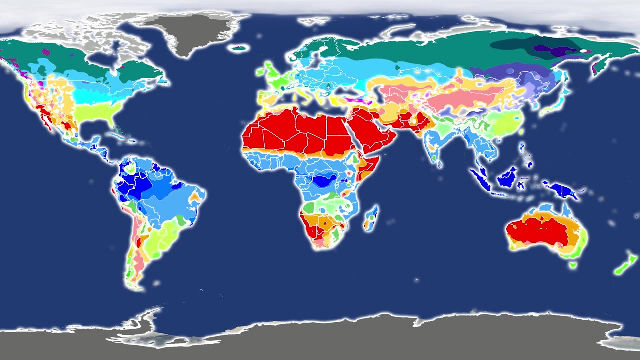 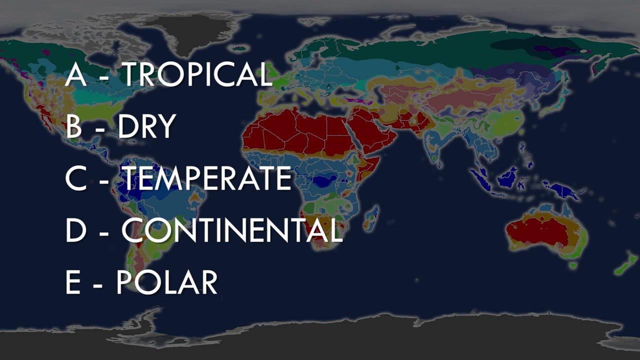 quick grasp of what on Earth I'm talking about. If you want to find a specific section, I've provided video bookmarks in the accompanying text. Overall, the Copen-Geiger system has five broad categories which describe a general pattern and roughly start at the equator and end at the pole. These are always the capital. 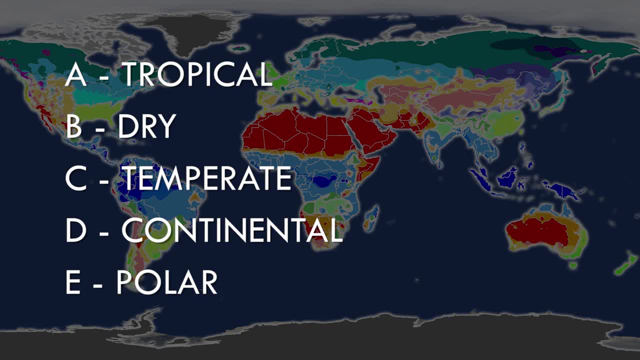 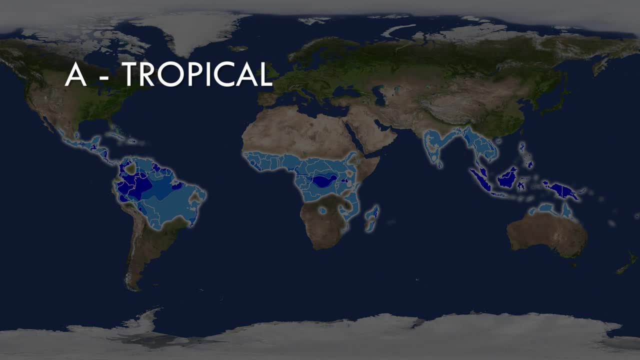 first letter of the shorthand codes that every Copen climate zone has, and are as follows: A – Tropical – the zones around the equator which are hot all year round and either have heavy rain all year round or during some part of the year. 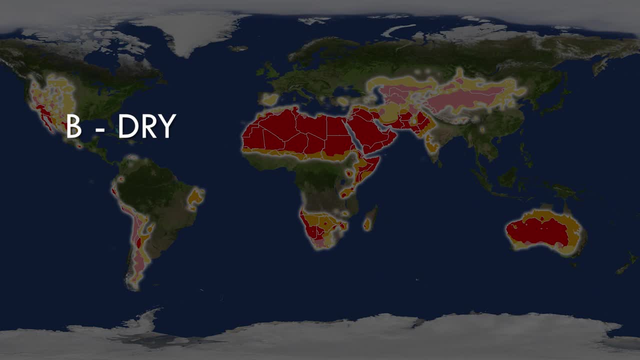 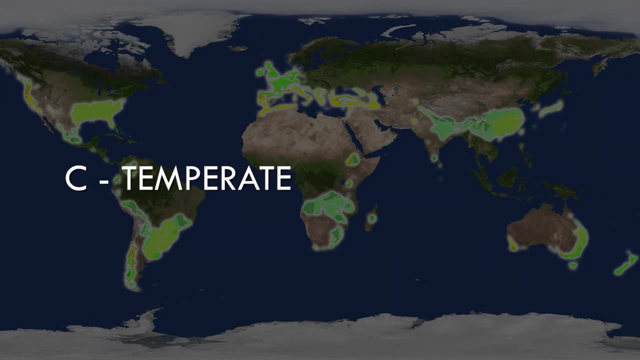 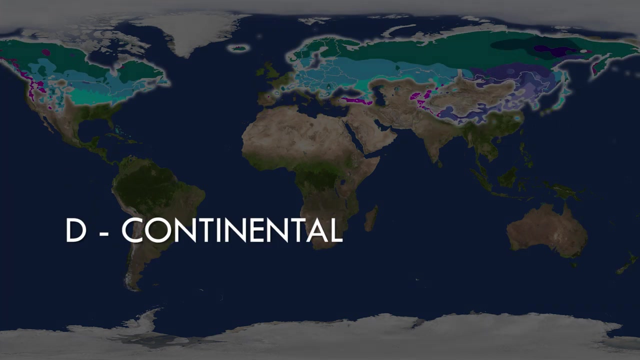 B – Dry – subtropical or continental areas with very little rain year round. C – Temperate – areas which have relatively mild temperature ranges year round and occurring at the mid-latitudes near the coasts. D – Continental – areas of high temperature ranges occurring usually deep within the northern. 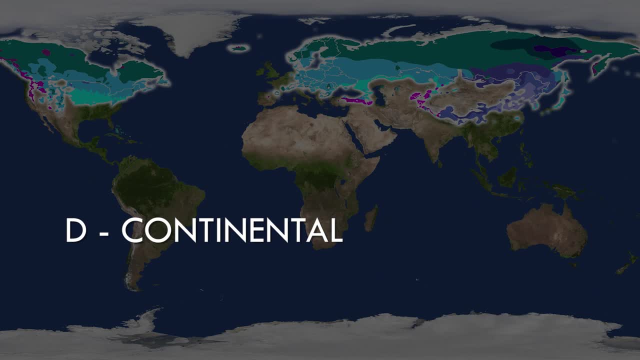 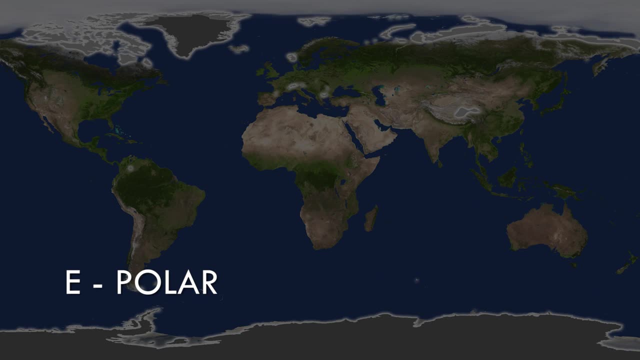 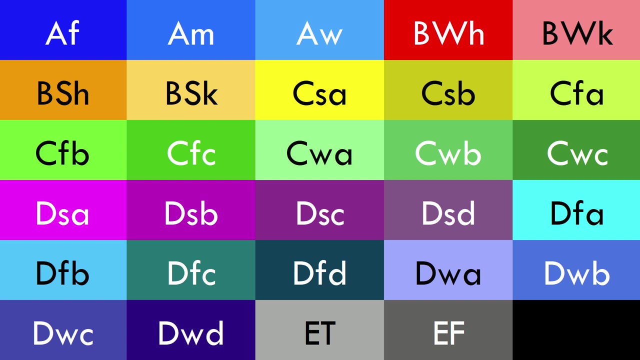 continents experiencing cold or very cold winters. E – Polar – areas which are cold all year round, occurring near or at the poles of our planet. Each of these broad categories is further subdivided to account for more precise differences in temperature or rainfall, and these give us the full two or three digit Copen-Geiger. 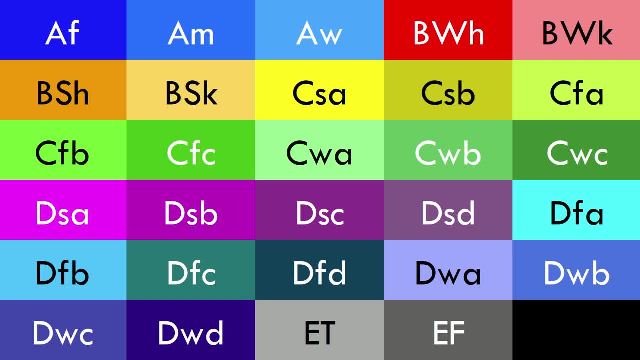 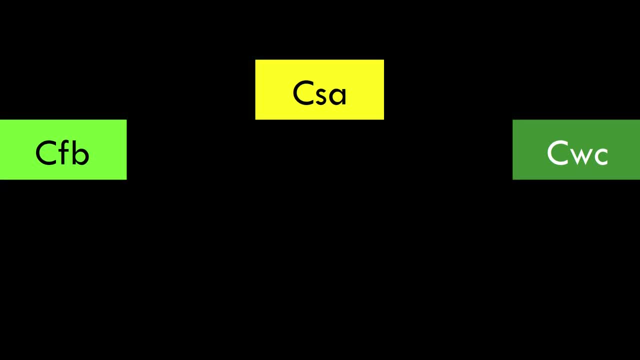 C – Continental – areas of high temperature ranges occurring usually deep within the northern Geiger codes. These codes at first might seem like they're just hieroglyphics, but a quick look can reveal the logic on 80% of them In all the temperate and continental codes. the second letter tells us when there is a dry season. 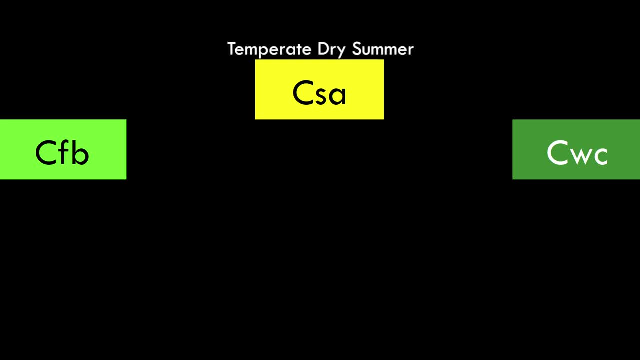 S means the dry season is in summer, W the dry season is in winter And F for no dry season at all. The third letter tells us how warm or hot it is, with A being the hottest and D being the coldest. 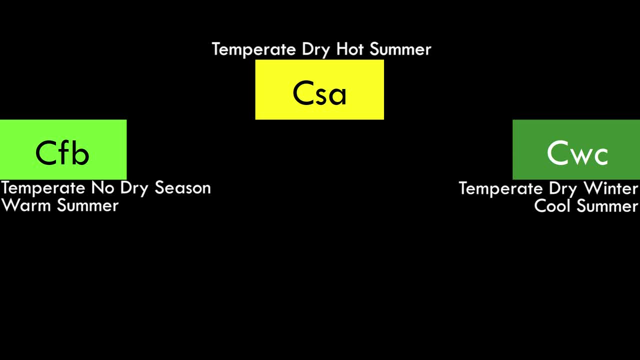 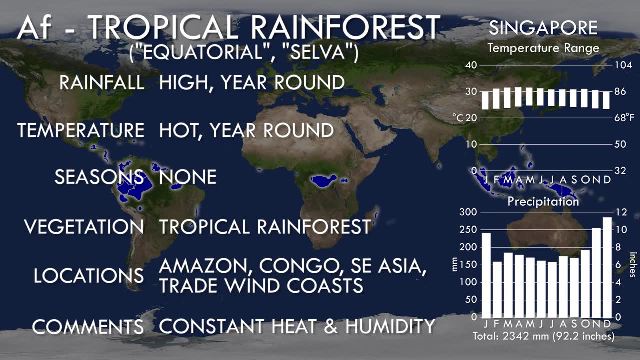 So, armed with this knowledge, let's get straight into looking at each and every one of the Koppen zones AF: the tropical rainforest, also known as the equatorial climate, or salva, which is Spanish for jungle, Occurring only within the tropics at low elevations. 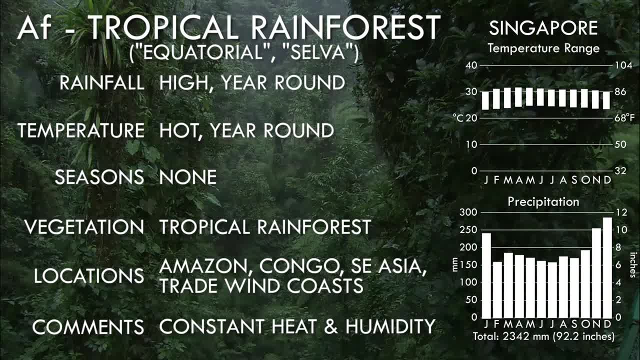 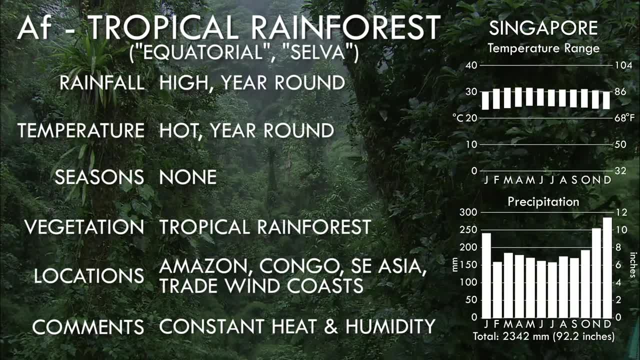 the key defining characteristic of this climate is rain and hot temperatures all year round. This produces the famous rainforest that the zone is named after and has the largest biodiversity on Earth, AM, the tropical monsoon Found also exclusively within the tropics. 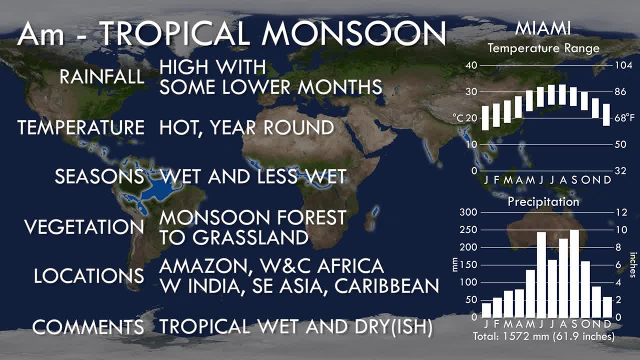 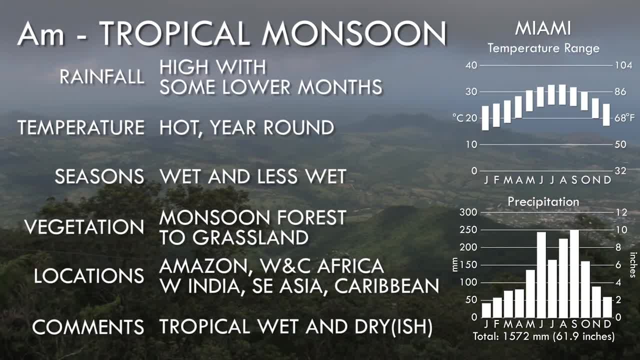 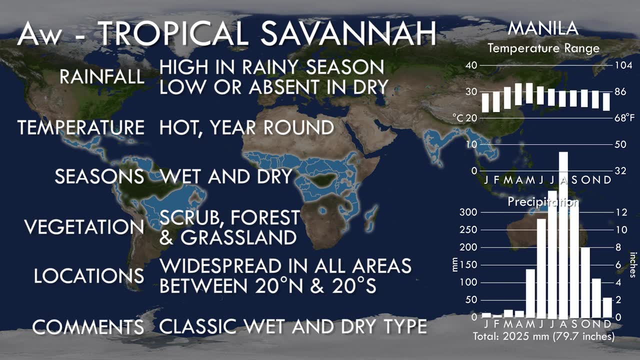 this climate zone experiences heavy rain during part or most of the year, but also has a relatively short dry or longer drier season due to the shifting directions of trade winds from land to sea and vice versa. AW- tropical savannah, A close sibling of the tropical monsoon and covering a much larger area in the tropics. 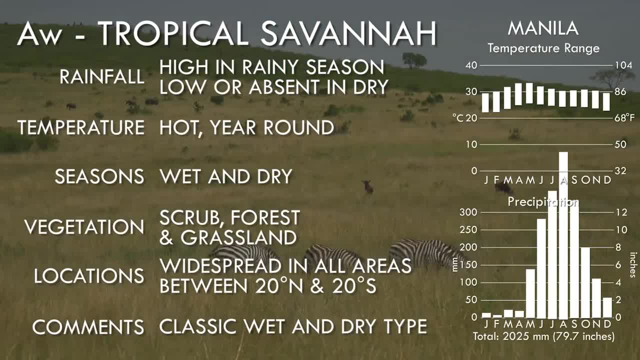 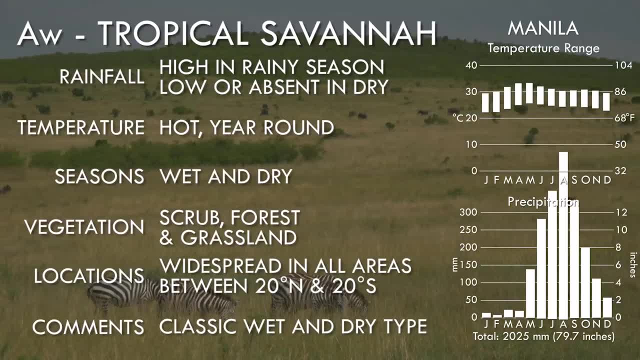 here, the dry season is either completely dry or is dry over a longer period of time. Both the savannah and the monsoon have a mix of woodland and grassland, depending upon the amount of rain and local topography. Both support enormous populations and many large cities. 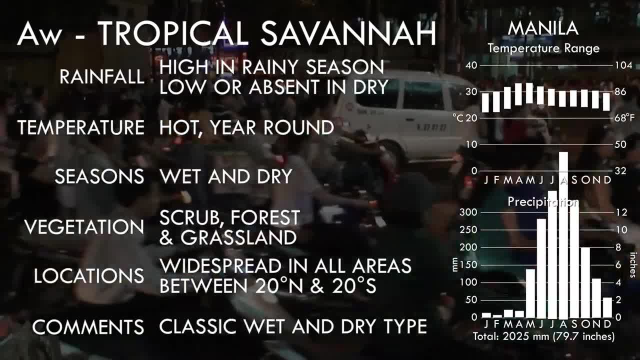 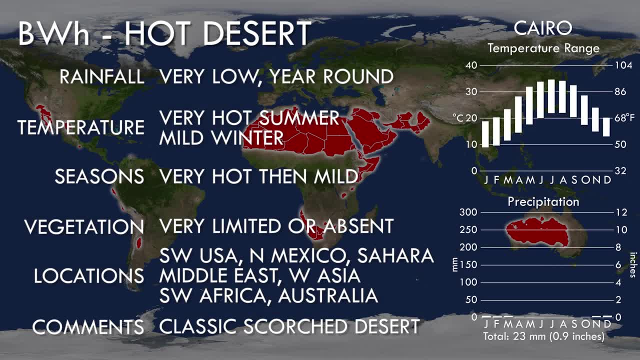 due to the combination of heat and rainfall, without the human health issues of the rainforests. BWH- hot desert. Lying on the border of the tropics, these areas experience very little rain and searing summer temperatures, which hold the records for the highest on Earth. 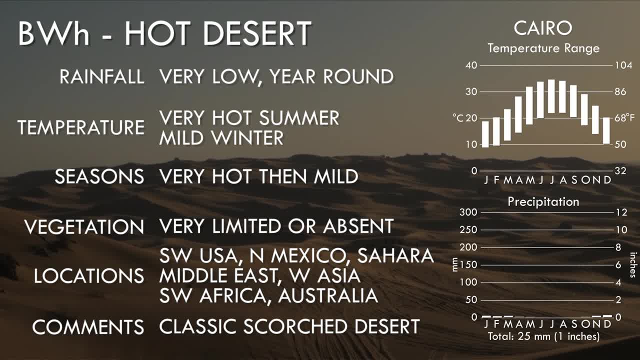 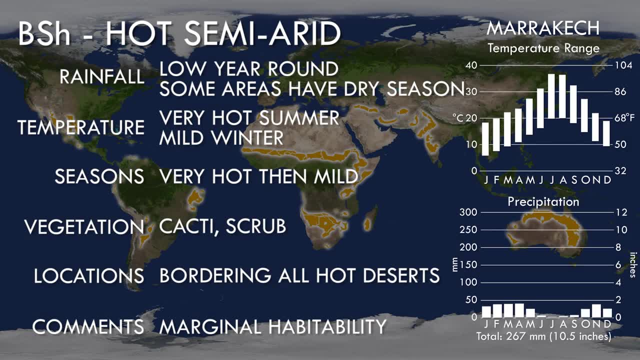 Little or no vegetation exists in the tropics, but it's not a problem. BSH: hot semi-arid. Lying next to hot deserts, these areas have a little more rain to support scrub-like vegetation, but are still marginal in terms of sustainable human settlement. 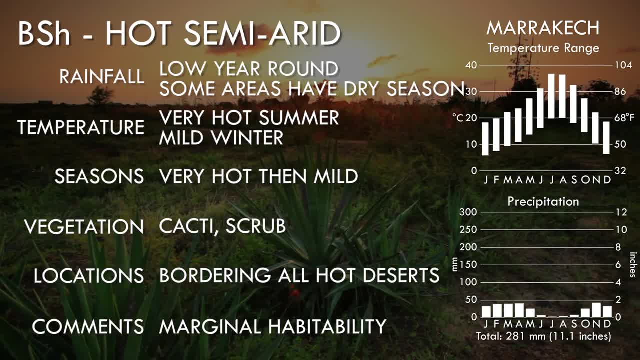 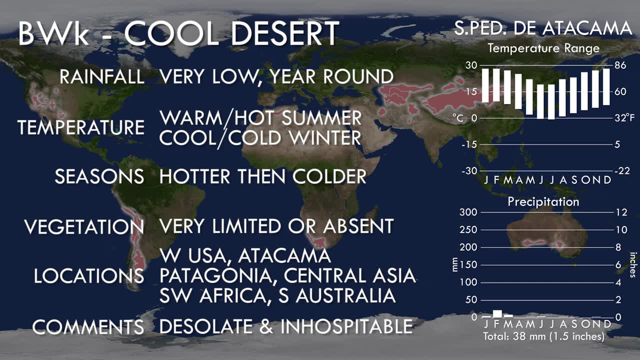 BWK cool desert. Lying deep within the continents, far from the ocean, or on the leeward side of mountains sheltering them from moist winds, these areas are as parched and desolate as the hot desert BWK cool desert. 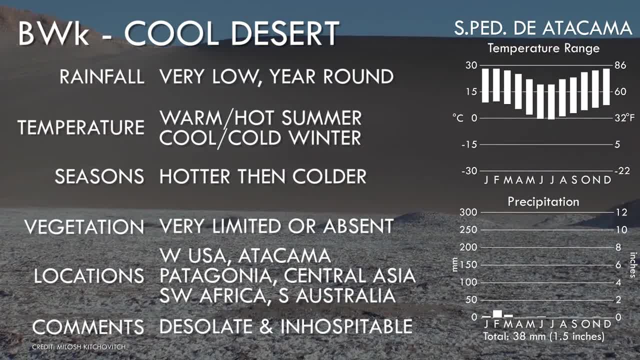 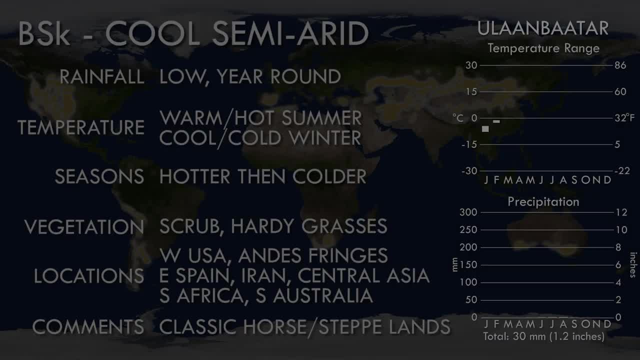 Lying deep within the continents, far from the ocean or on the leeward side of mountains. these areas are as parched and desolate as the hot deserts, but experience winter temperatures that often fall below freezing point. BSK: cool, semi-arid. 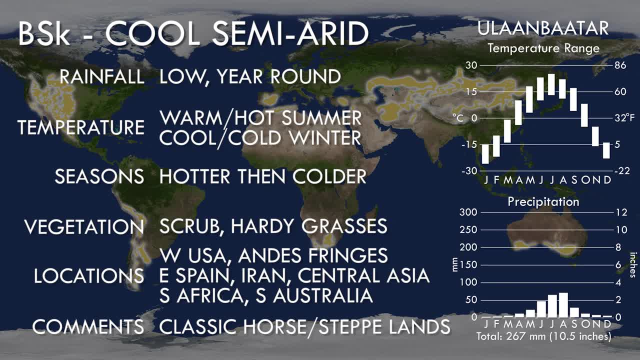 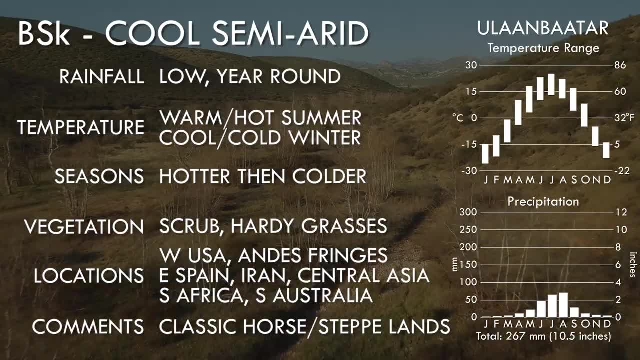 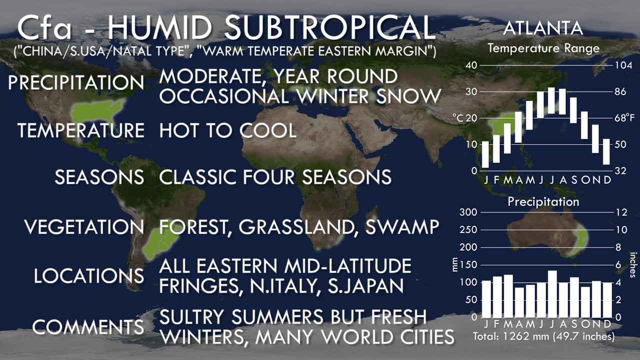 Like the cool deserts, only with more rain, but not enough to be classified as temperate or continental. Like their hot, semi-arid counterparts, they support shrub-like vegetation or hardy grasses. CFA: humid subtropical Lying at a similar latitude to hot deserts. 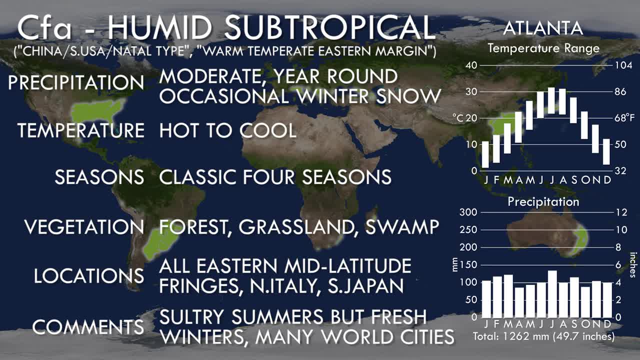 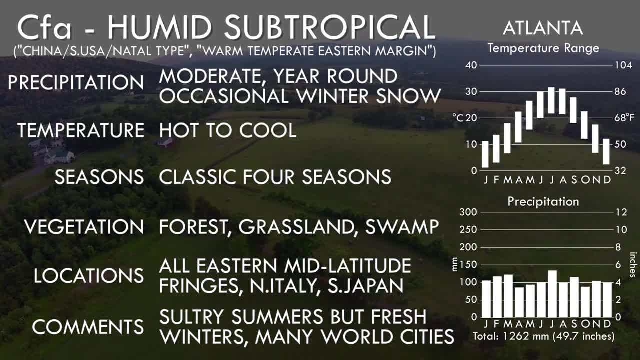 these areas are on the eastern fringes of the continents, however, and are next to warm oceans that bring in plenty of moisture. They experience tropical summers, but cool winters and rain all year round. They are amongst the most important areas of human civilisation. 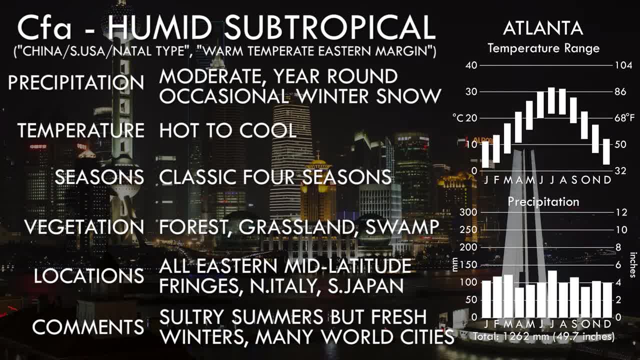 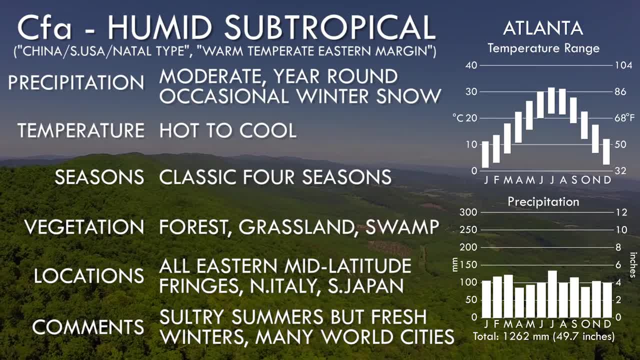 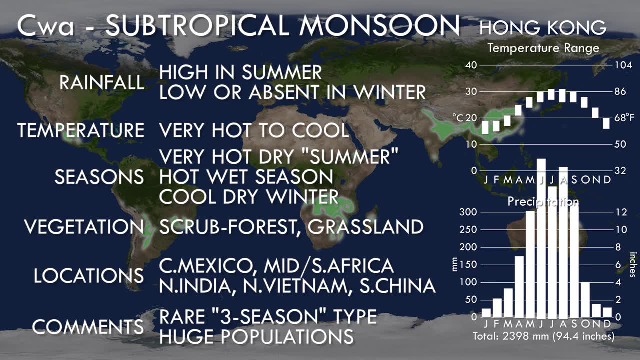 housing enormous populations and many great world cities. Typical natural vegetation ranges from the forests to swamp and grassland, but much of these areas have been given over to farming. CWA- subtropical monsoon, A sibling of the humid subtropical and found mainly in Asia at the same latitudes. 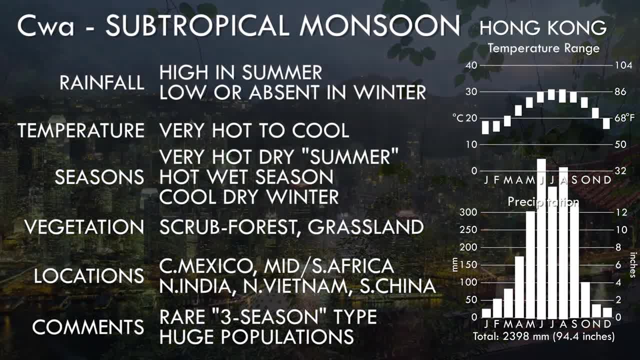 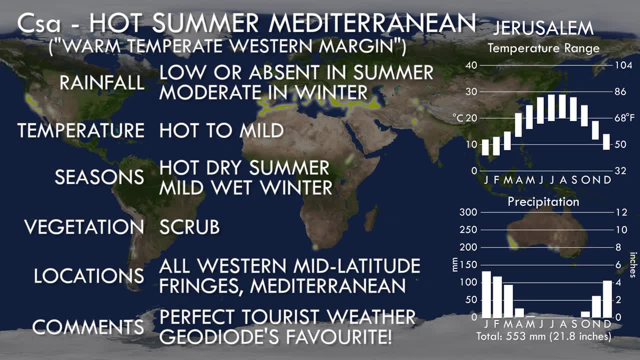 this varies only in that it has a winter dry season instead of the rain all year round, due to the presence of the Asian monsoon CSA, hot summer Mediterranean, Lying just above the hot deserts in latitude and always on the western fringes of continents. 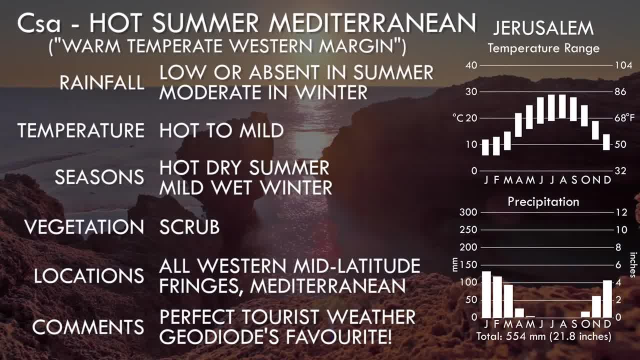 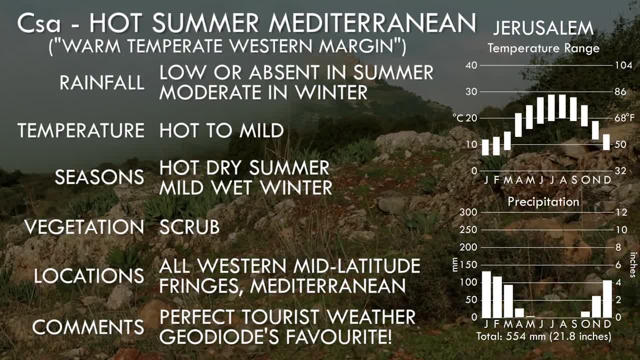 these areas experience the hot and dry conditions of deserts in summer, but significant rain from oceanic westerly winds in winter. Natural vegetation is limited by the desert-like conditions of summer and is typically shrub-like. CSB- warm summer Mediterranean. 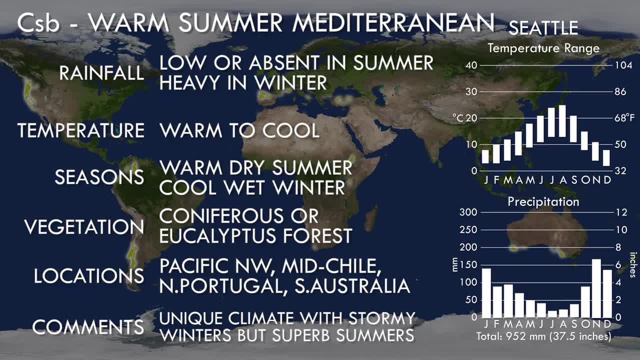 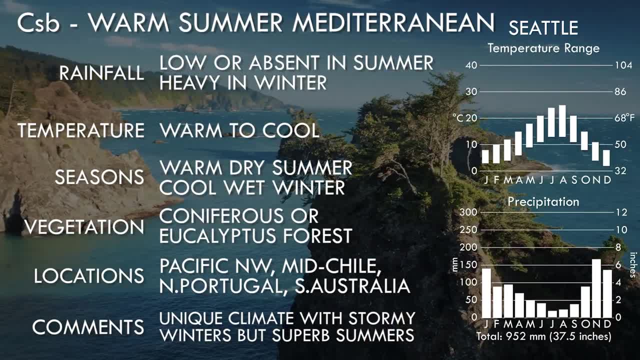 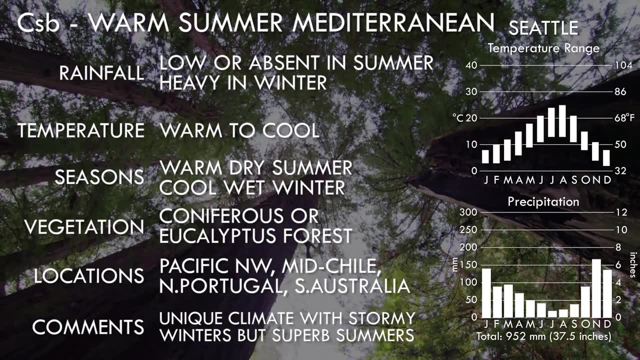 Always lying above their CSA siblings on the continental western coasts, these areas have warm, dry summers instead of hot and usually even heavier rainfall in winter, With less harsh summers. natural vegetation is usually in the form of coniferous forest, including the redwoods and sequoias of California, the tallest in the world. 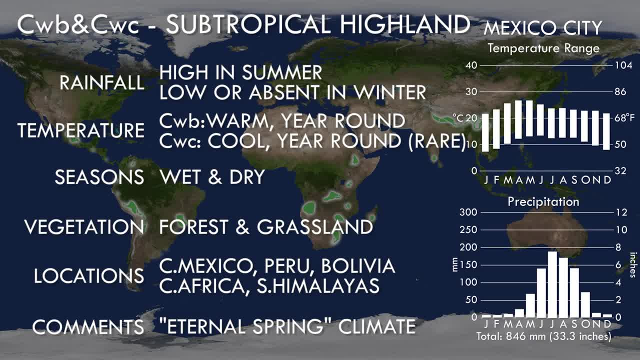 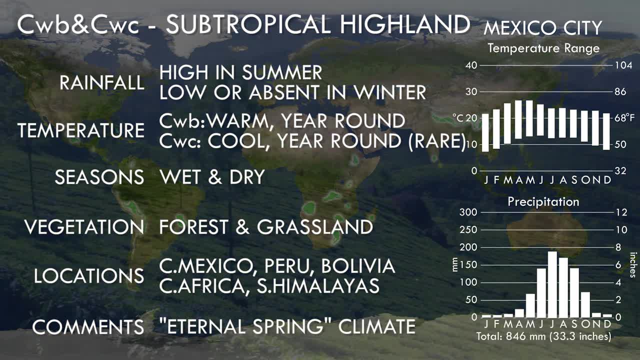 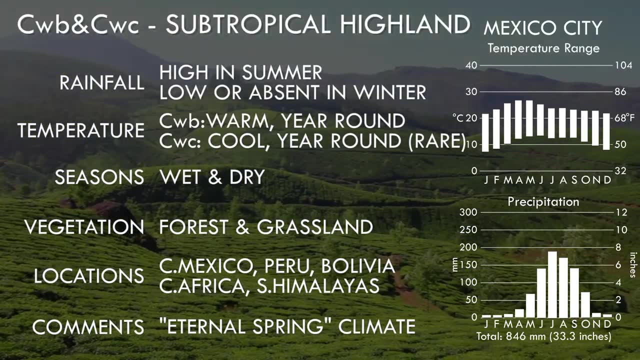 CWB subtropical highland Occurring in tropical latitudes. the heat of the rainforest and savannah is reduced significantly through being at high altitude. The result is year-round mild temperatures with a pronounced dry season, Found mainly in Latin America, East Africa and the foothills of the Himalayas. 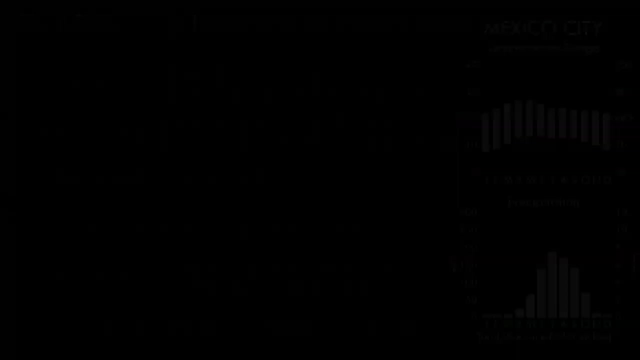 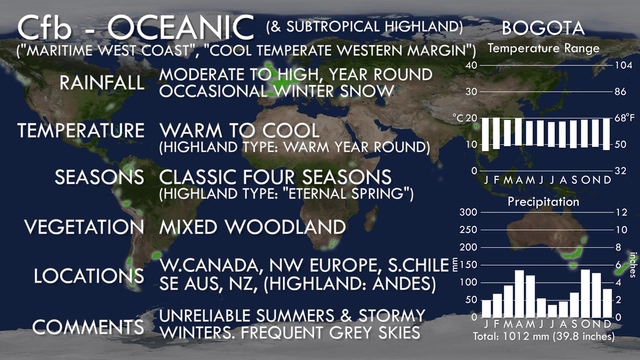 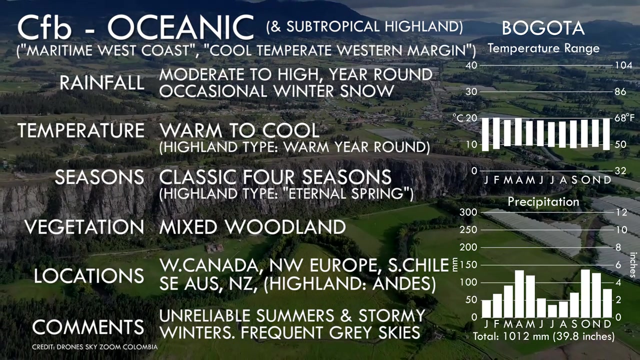 natural vegetation is a mix of forest and grassland. CFB: oceanic and subtropical highland. One of the more confusing cop and codes, the CWB Due to an accident of nature, creating very similar conditions for completely different reasons. Small upland areas near the equator, such as in Colombia and Ecuador. 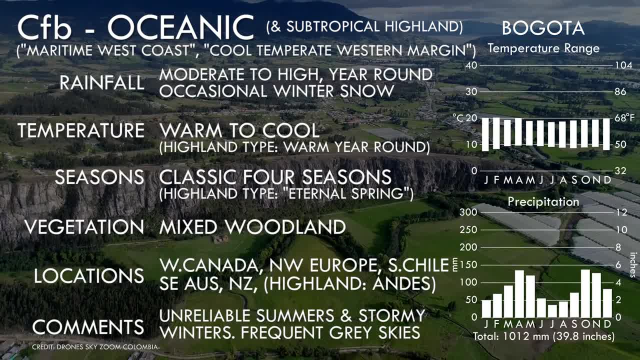 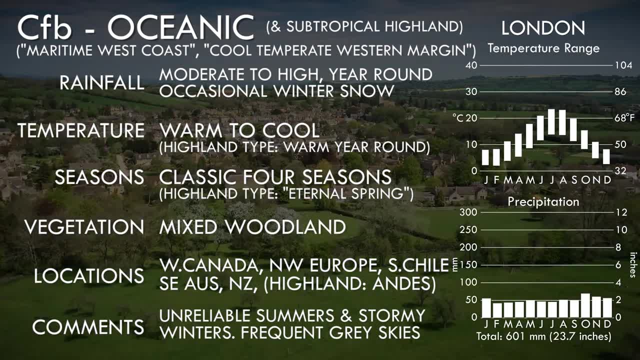 have this mild year-round climate, which also experiences year-round rain, But over much larger areas in the mid-latitudes. this climate exists next to western coasts, where prevailing westerlies moderate temperatures year-round, such that warm summers and cool winters are the norm. 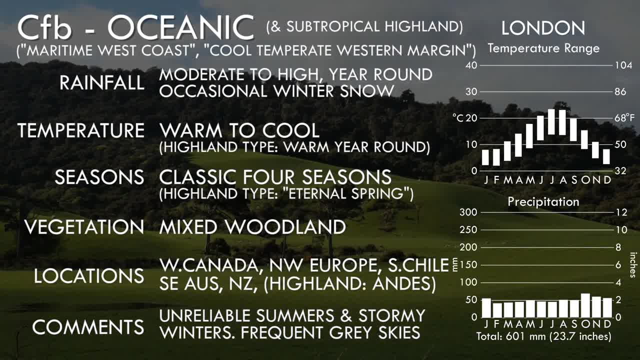 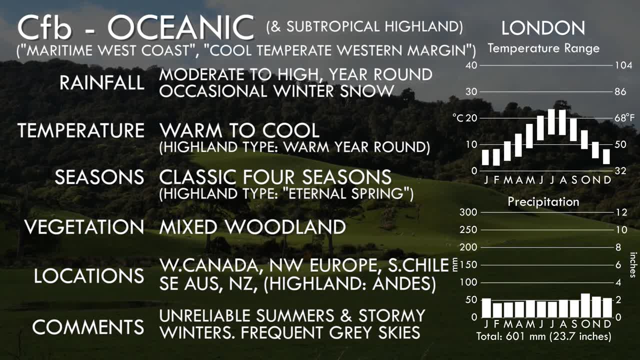 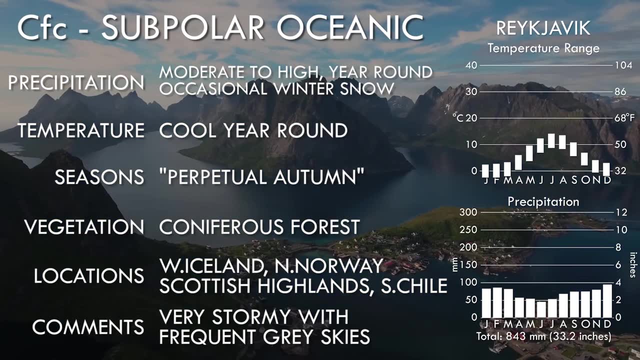 In both cases, limited seasonal temperature range and year-round rain are its defining hallmark. Natural vegetation is mixed woodland, but these areas are heavily farmed. CFC, subpolar oceanic, Lying in certain areas higher in latitude or elevation to the oceanic. 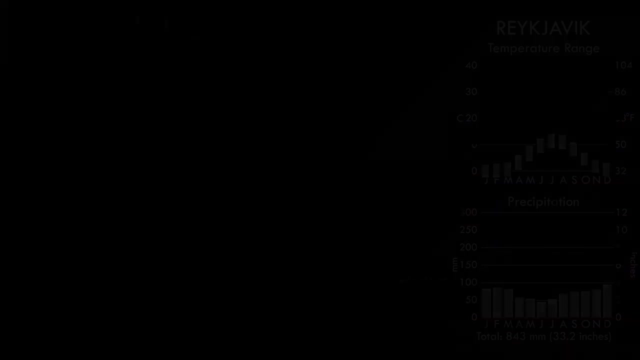 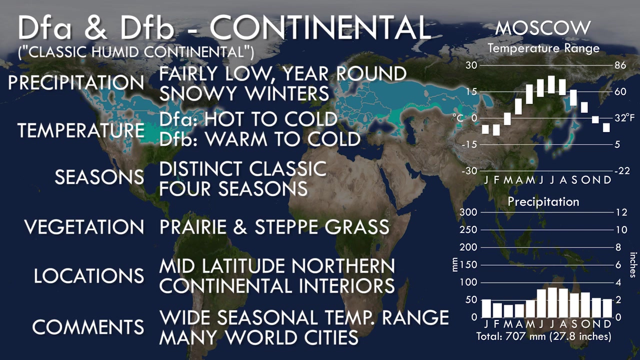 these areas still have mild winters but cool summers. DFA and DFB: The first of the six continental climates occurring only within the great landmasses of the northern continents. All these climates experience high temperature ranges between summer and winter, and all have cold winters, routinely falling below freezing. 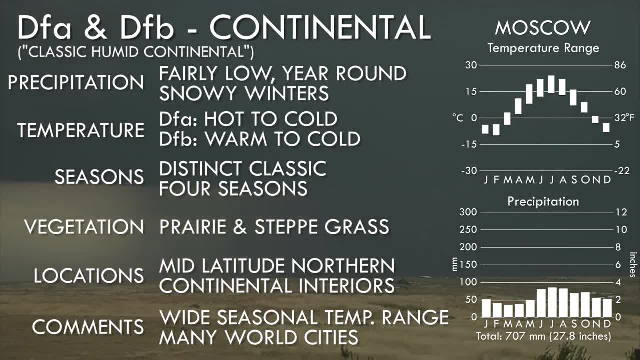 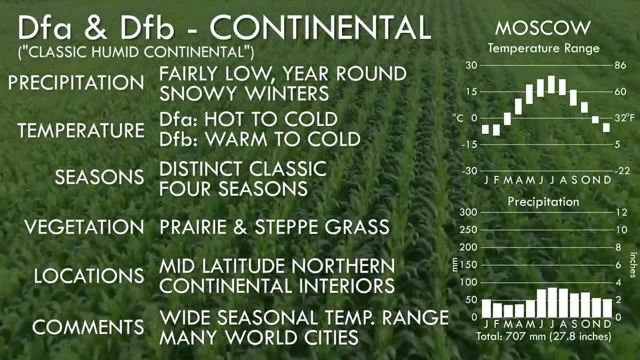 These first two experience rain year round, with DFA experiencing hard summers and DFB experiencing somewhat cooler but still warm summers, and are the most prevalent occurring across wide continental areas. Natural vegetation is usually in the form of grassland, but these areas are heavily farmed. 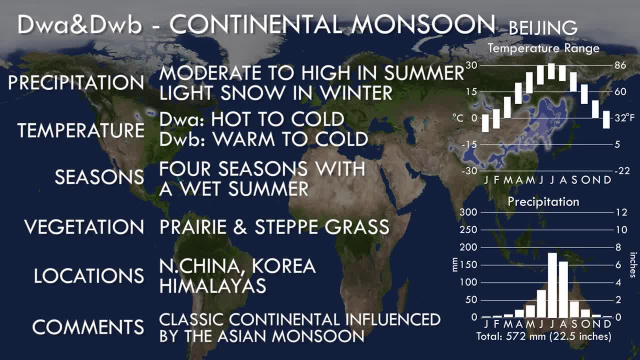 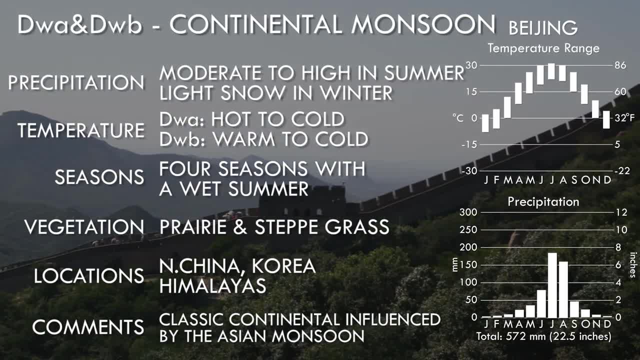 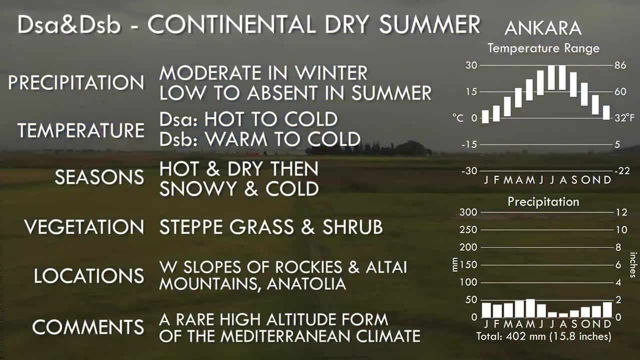 DWA and DWB, The same as DFA and DFB, except that there is little to no rain during the winter. These occur exclusively in Eastern Asia due to the influence of the Asian monsoon. DSA and DSB: The same as the other continental climates, except that the summer is dry instead. 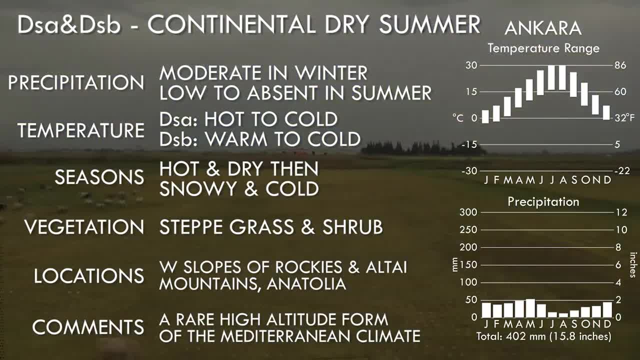 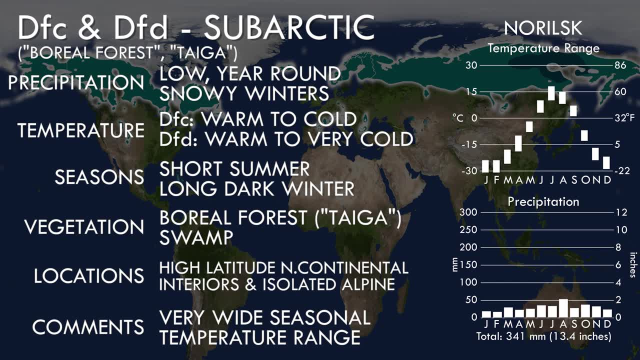 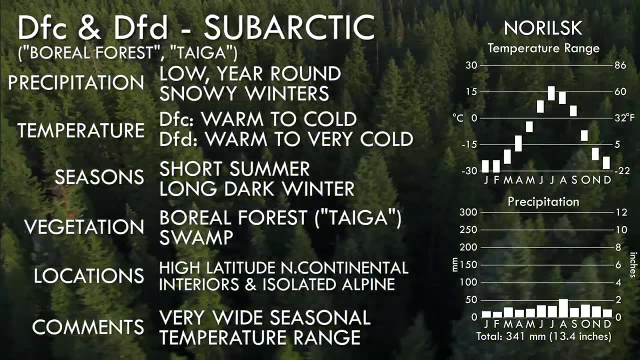 of the winter. These areas are not common and usually occur inward from Mediterranean climate areas DFC and DFD, The first of the six sub-arctic climates. These areas, lying to the north of and similar to the continental climates, except winters are much, much colder. These two zones have rain or snow year round, Like all the. 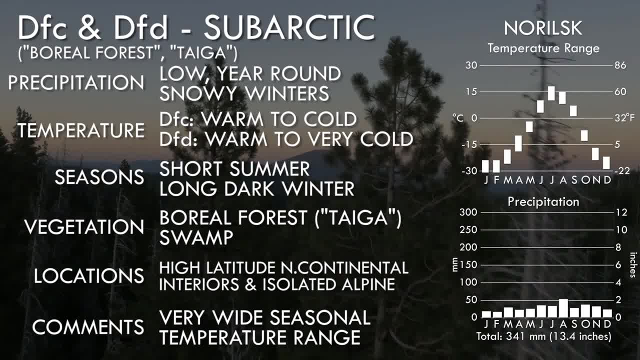 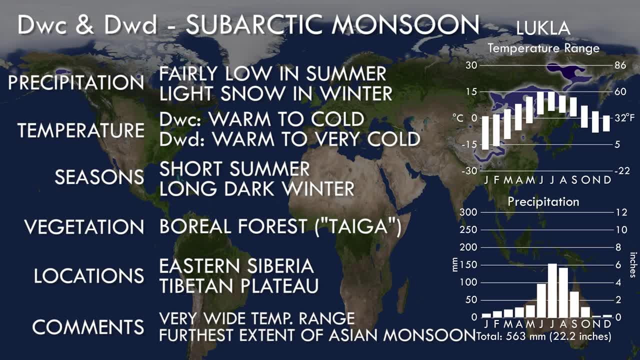 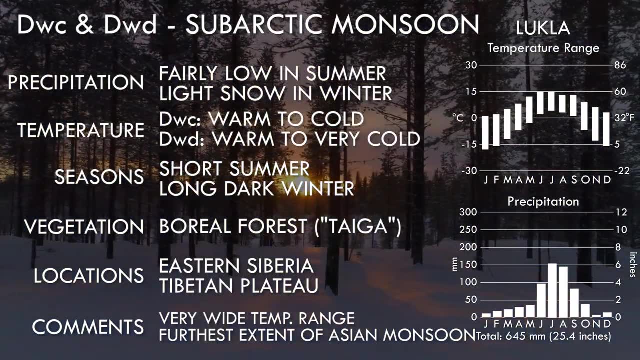 sub-arctic zones. the vegetation is dominated by coniferous forest, known by the Russian word taiga, and farming is almost non-existent. DWC and DWD: These sub-arctic zones are identical to the first two, except they have dry winters. They occur only in Eastern Siberia. 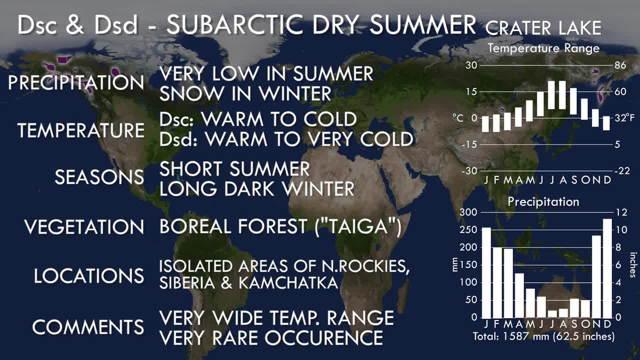 DSC and DSD. These very rare sub-arctic zones. are very rare sub-arctic zones. These very rare sub-arctic zones are very rare sub-arctic zones. These very rare sub-arctic zones. are very rare sub-arctic zones. These very rare sub-arctic zones. 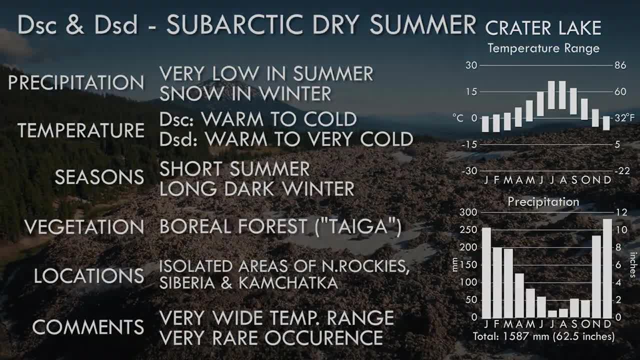 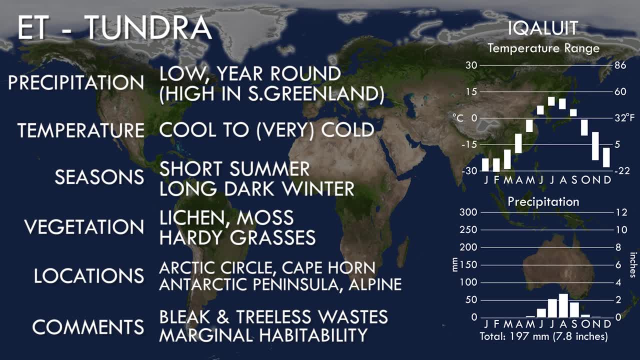 are like the others, except that the dry season occurs in summer. ET Tundra. Even further north than the sub-arctic, the true arctic has the treeless waste of the tundra, where summer temperatures are just too cold to support tree growth.